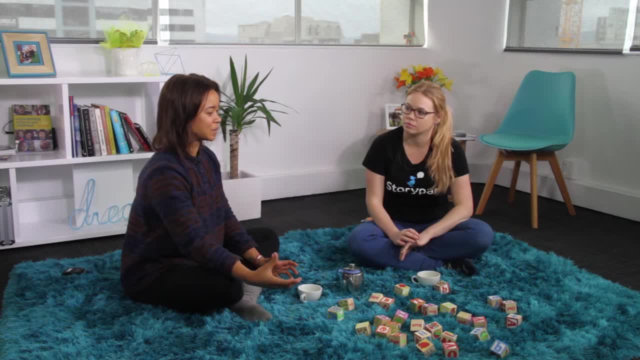 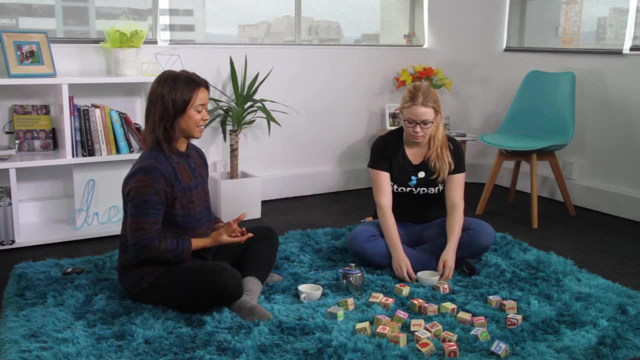 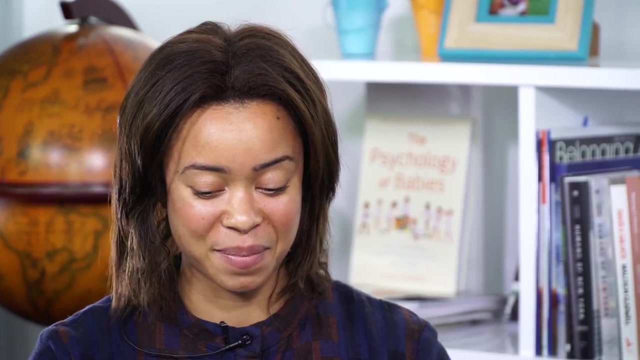 of teaching yoga with the women, But it was children that gravitated more towards the yoga, because I think the women just had so much going on in their minds that they had other things to deal with. And it was just all these children just roaming around the refugee camp And it was just 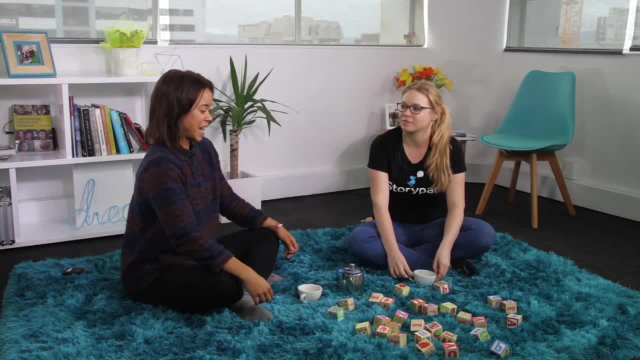 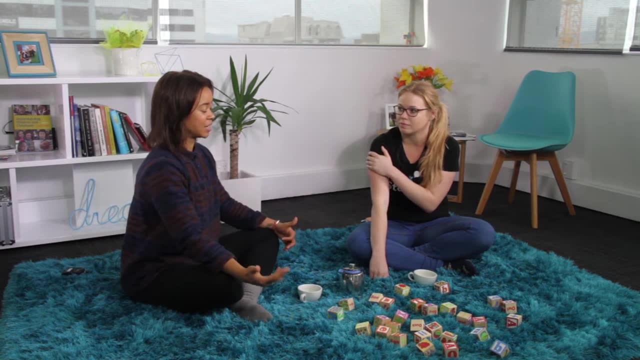 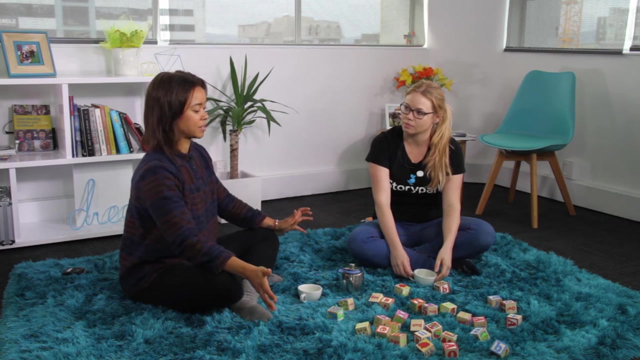 such a great experience, Like it was just just having fun and moving in different poses and kind of getting off their minds, off of like what will happen, Will they seek a solution, Will they seek a asylum, Will they go back- And I thought it was very useful to create a mindful practice. 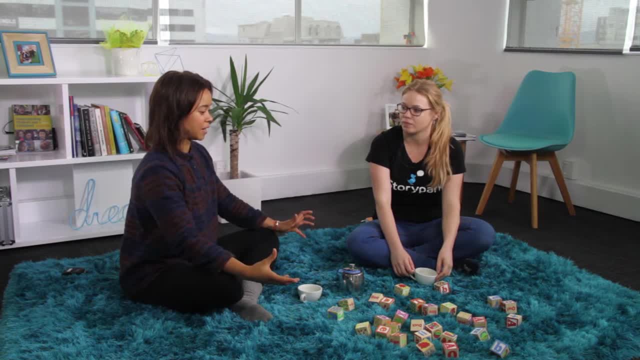 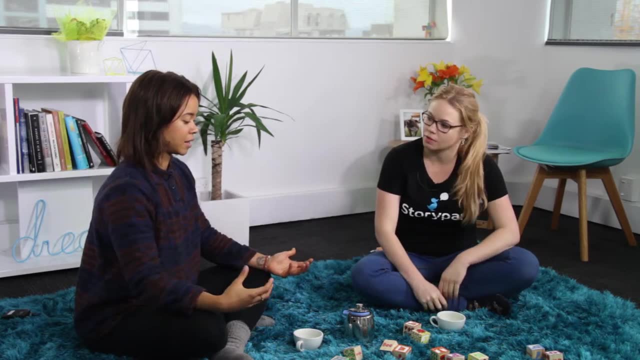 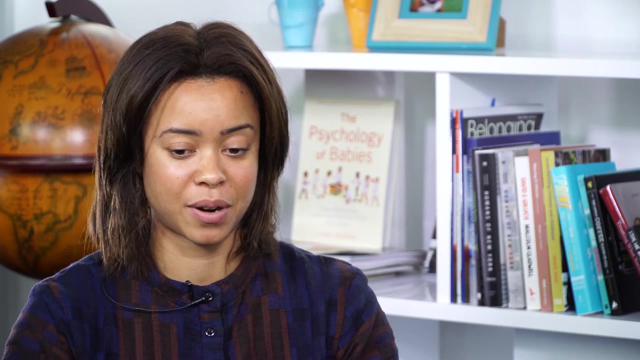 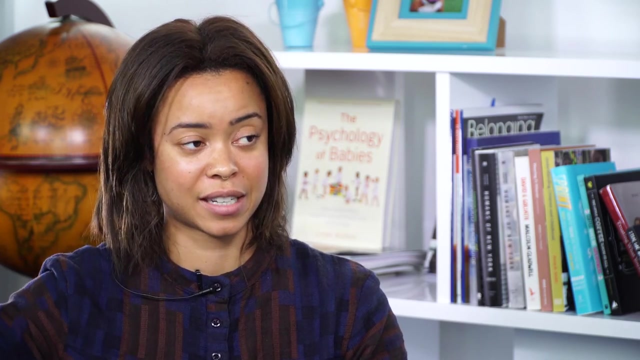 for the children to just kind of get their minds off of where they are and what the situation is. So, especially for children with trauma, I think, getting that mindfulness in terms of breathing, staying present and kind of allowing all that excess and all the excess to kind of just come down and bring it back down and creating 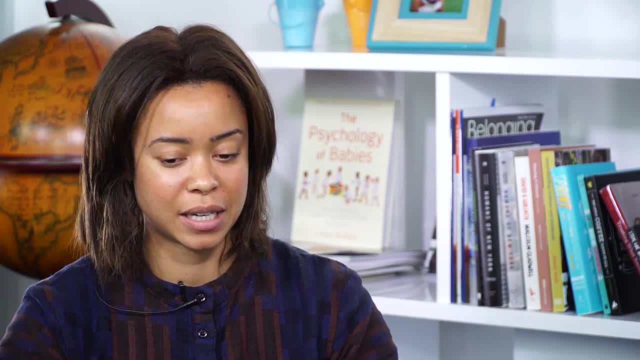 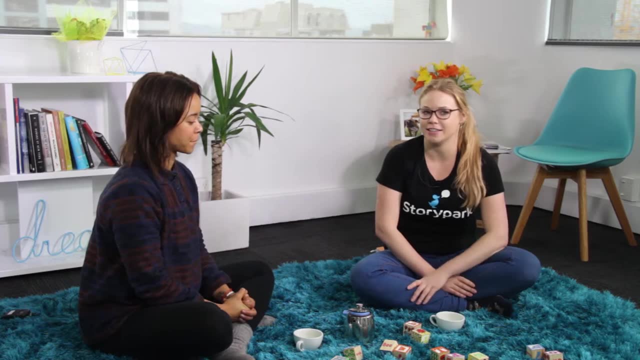 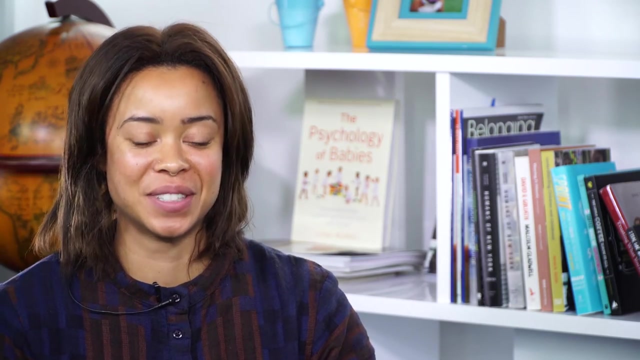 a more homeostasis and harmony. what are the challenges of teaching yoga to children? I imagine it's. there are a lot of differences between teaching to adults as opposed to children. yeah, I think you come into it not expecting the same thing you would would with adults. you're not necessarily looking for a 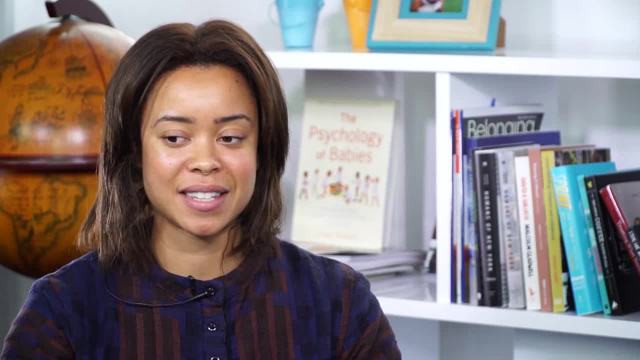 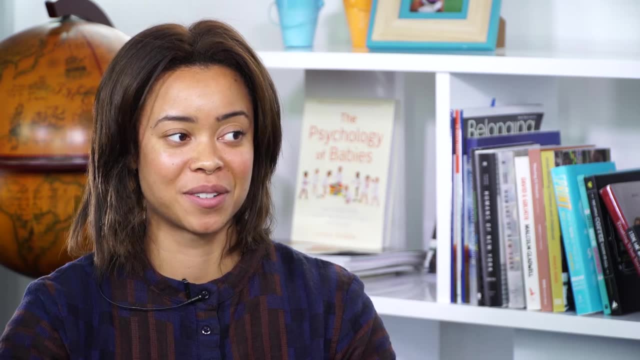 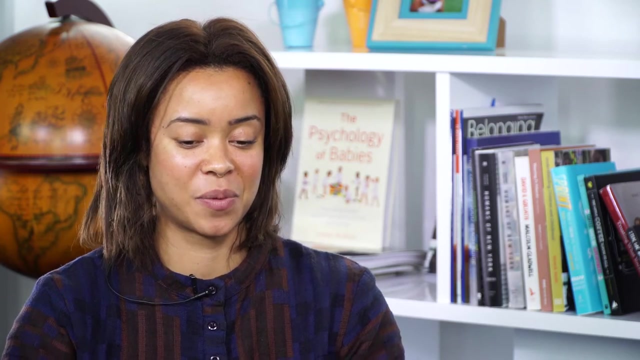 long string of focus. and especially- I say it's the same thing- when you come into a new meditation practice. some days it's easier and some days it's harder, depending on the energy level. it's as of being patient, knowing that the attention will be there and then all go, and you know when we're in a meditation practice. 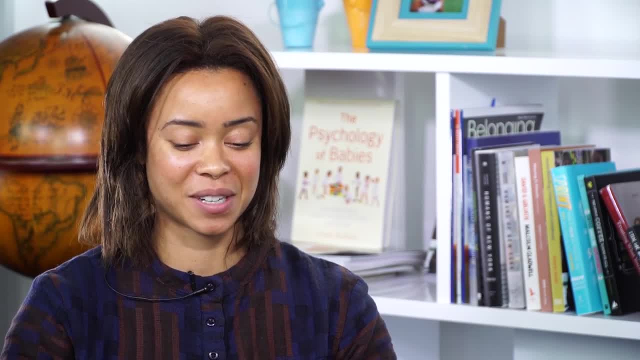 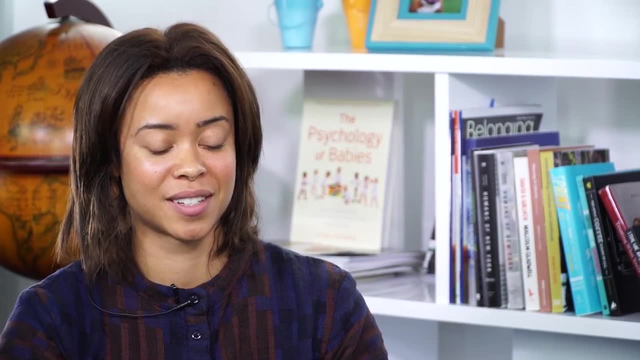 like we're being meditative, we're focusing, focusing on our breath, but then something else comes up and and it's just kind of understanding the fluctuating fluctuations of our mind. so if you are teaching a yoga class with children, is it typically shorter than what you're teaching? 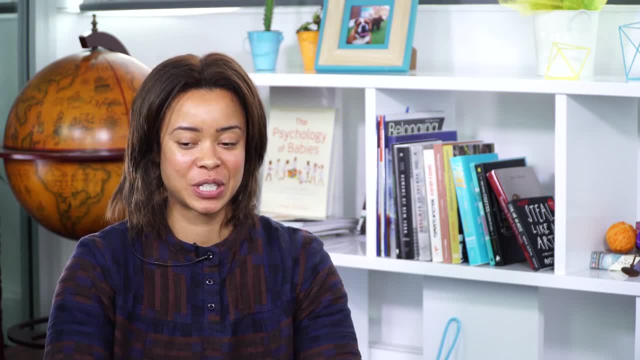 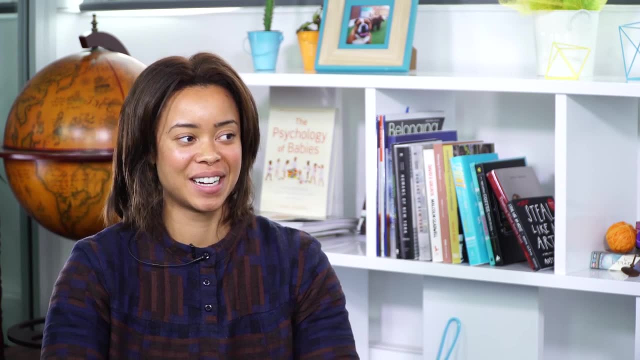 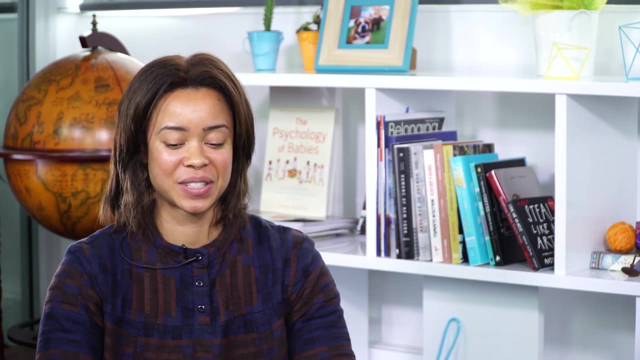 exactly. it's like: oh, it's shorter, and knowing that one kid might stray off or they might just like watch, or you know, so it's just kind of allowing, and then eventually they'll start to get it, you know. so it's just kind of not coming. 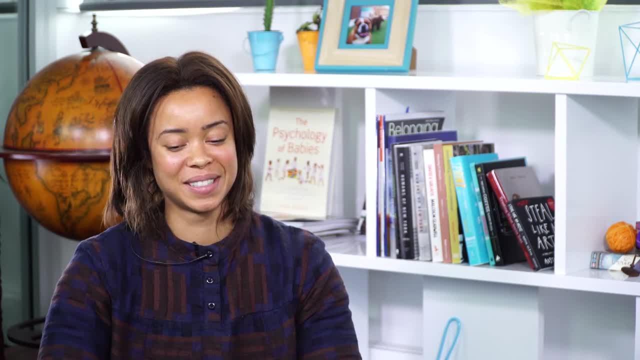 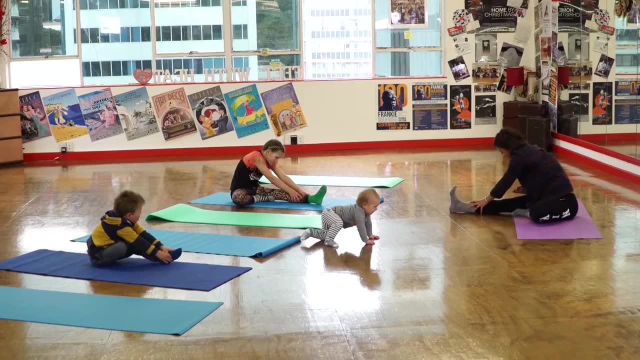 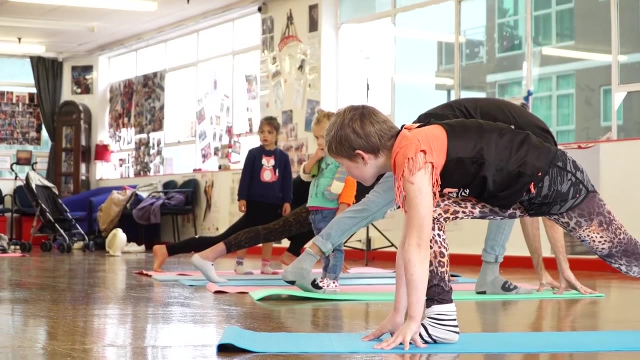 with any real rigid guidelines, but knowing that the message will eventually start to come across. yeah, so, like earlier, when we were doing that yoga, there was some kids joined in for part of the time and they wandered off. some decided they actually wanted to run around and that you just carried on. is. 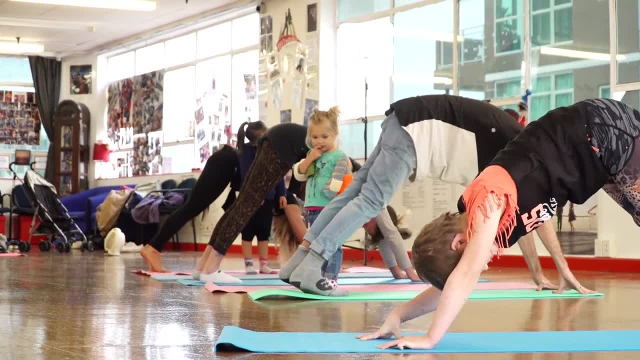 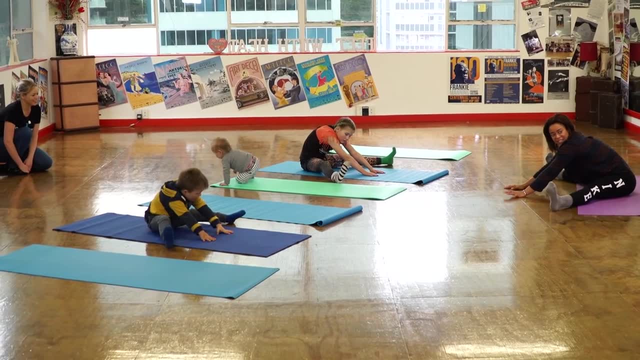 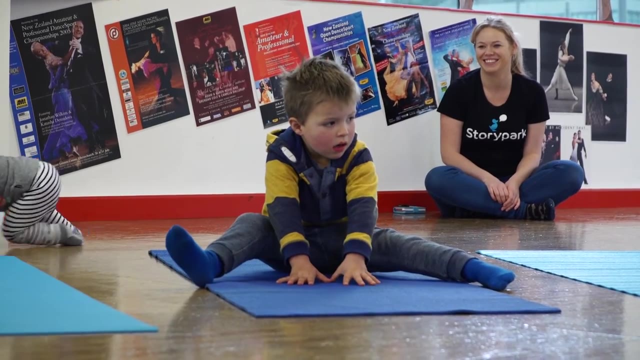 that quite typical of a yoga class with children, absolutely, it's totally typical. and eventually I think they start to understand like, oh, like I feel my breath or I feel it's kind of like in the beginning we're like: you have nap times as children, right, and how nap like nap. 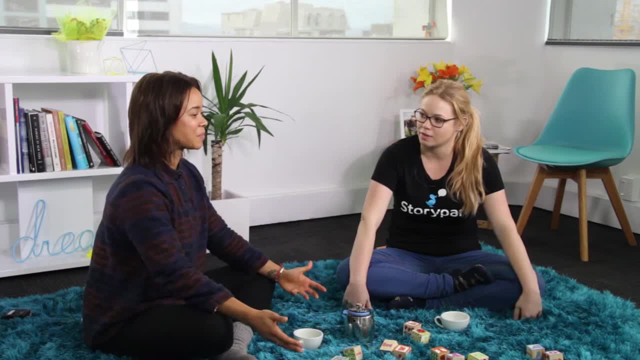 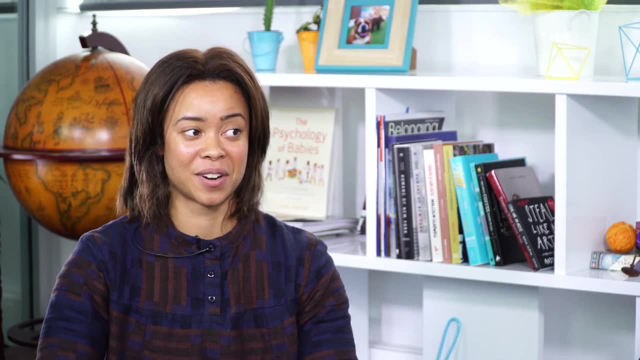 time kind of balance that out. it balances up the child. it could very much be like that for them. it's more introspective because they start to understand like, oh, when I go to yoga I feel like more calm. so do you think children can meditate? do you think maybe it's even? 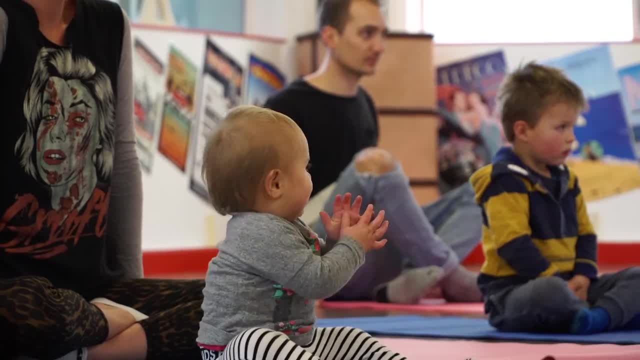 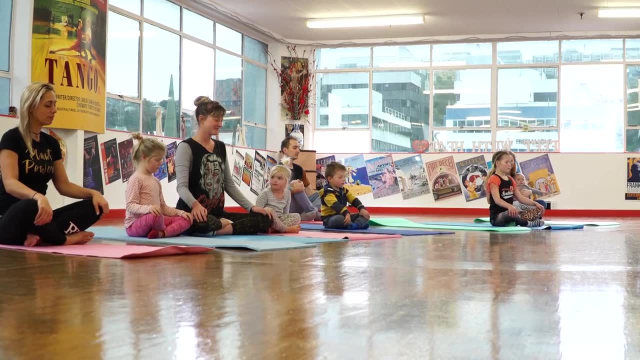 easier for them to, because as adults we don't know how to calm our minds. but perhaps it's different, exactly it's. I think it's so much easier for a child to pick up a meditation practice, in my opinion, in terms of like you never hear. 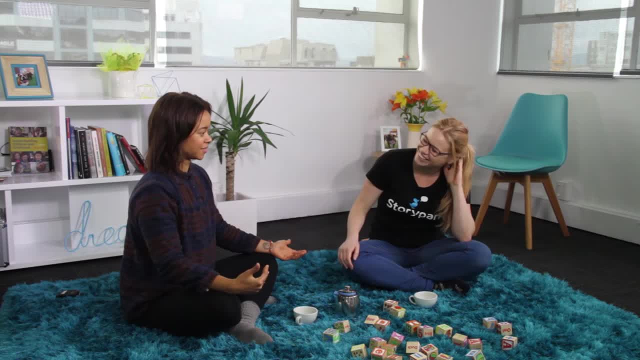 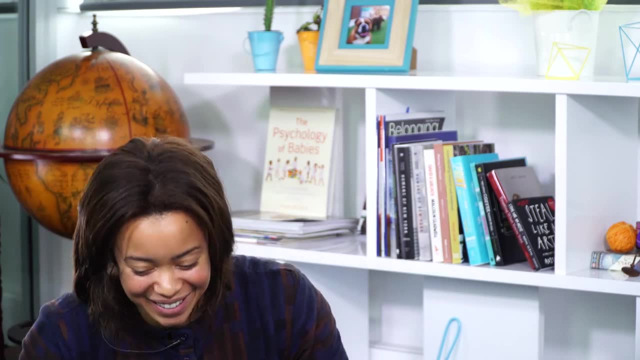 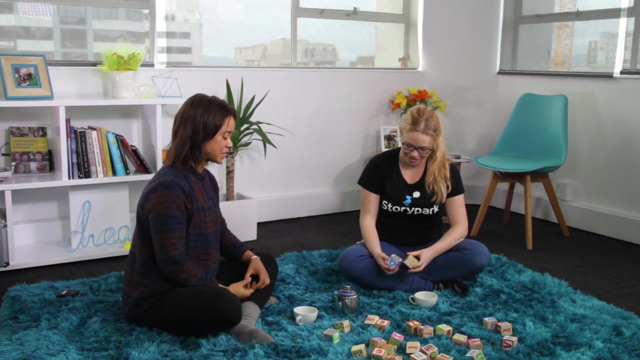 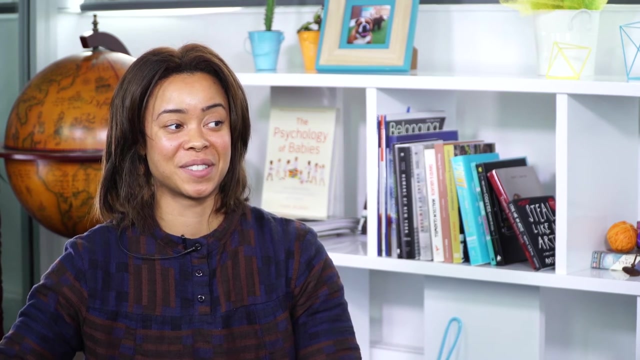 a child complaining of bad sleep. so much on my mind. so much starts to change as we get older, and if we had instilled those kind of practices when we were younger, things would be a lot different as we got older. you know, like I think we're living in the current time of like high stress and like the world is in a 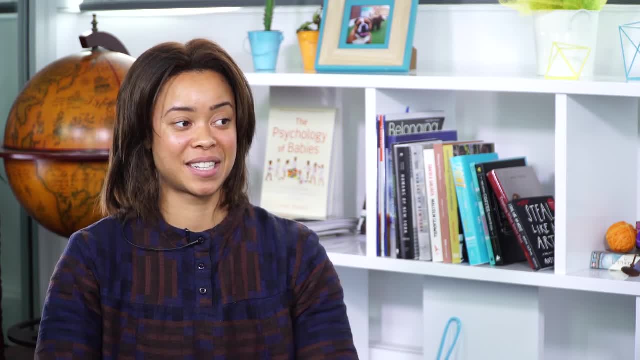 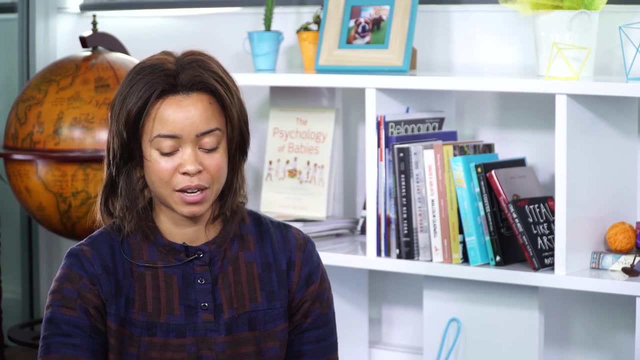 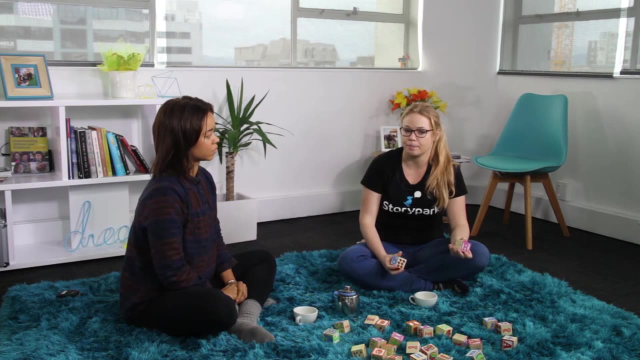 like you know, a very sensitive state, and I think the practice of yoga and the practice of meditation really allows us to be selfless and really allows us to see things for what they really are, without getting the ego too involved. something that I think other people as well as me might wonder about is with 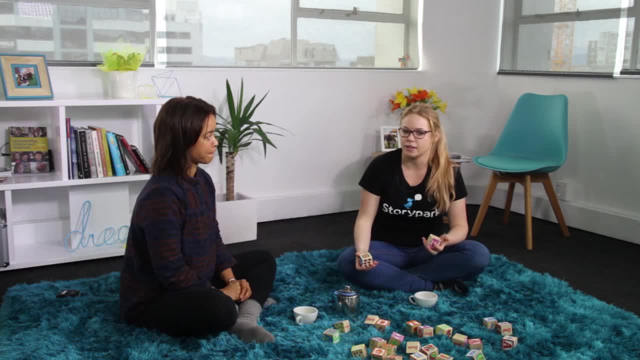 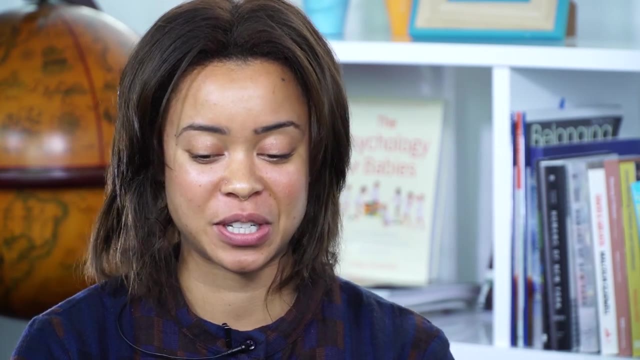 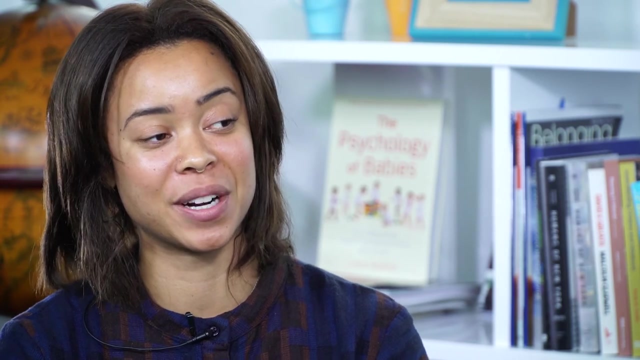 growing bodies is yoga. can it be bad for children to do yoga when their bodies are different and muscles are really changing all the time? no, and it's funny because when you start to look at the history of yoga, especially Ashtanga, it was actually for young boys, so it was a part. and in India, like the 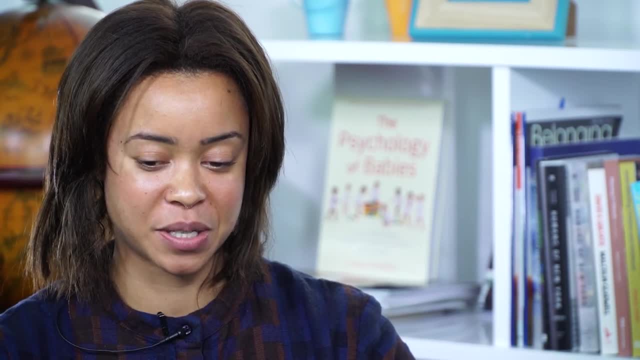 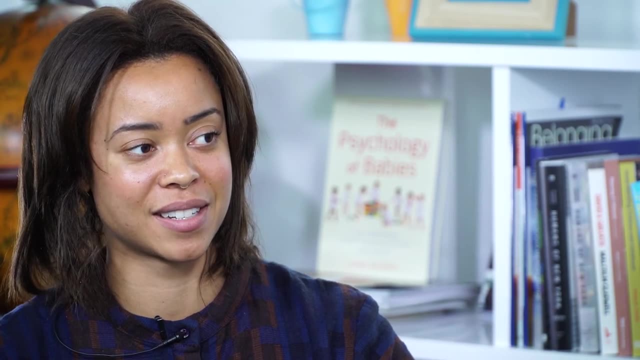 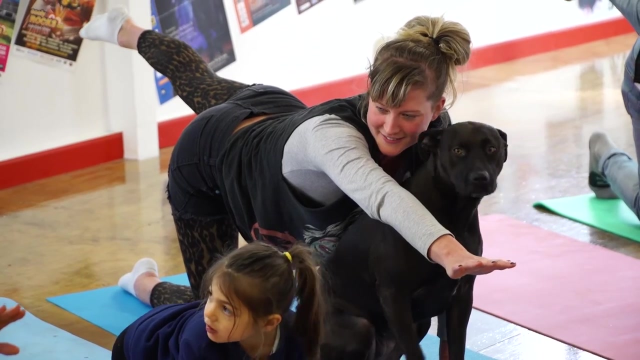 higher class were doing yoga right, and so the boys would on be having like very kind of like a lot of physical activity, kind of strict yoga practices, and they saw this of value. you can tailor a yoga practice to the individual. so no matter what the body shape, no matter what the 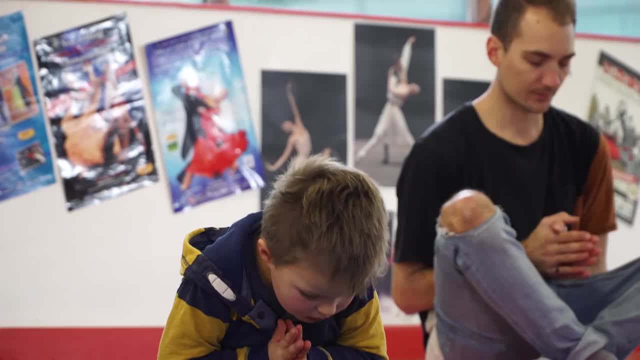 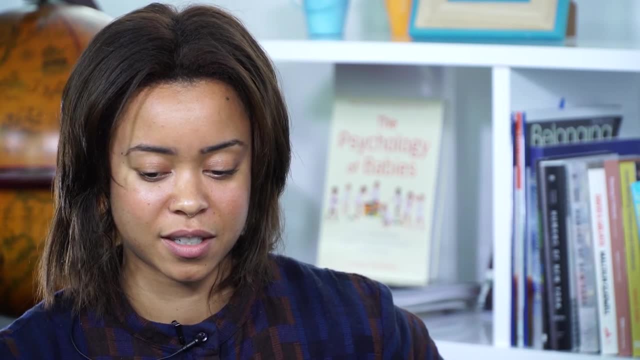 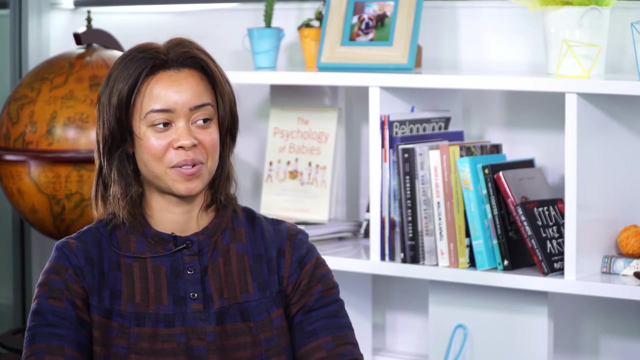 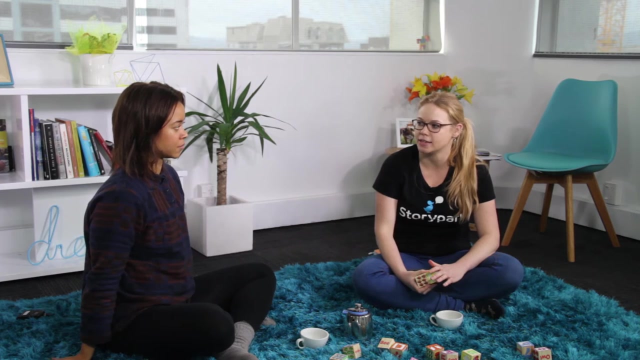 history. I think yoga is really just the yoking, the union of the mind. so whenever there's movement with breath, that's yoga. sitting here, closing your eyes and observing the qualities of your breath is yoga. Do you have an example of a pose that you would teach to children and the shape it would make and and how, how you would teach it? 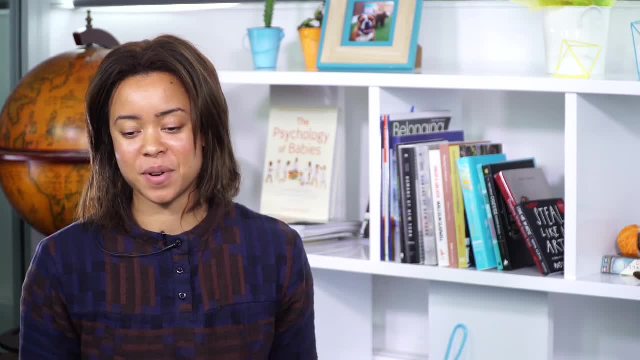 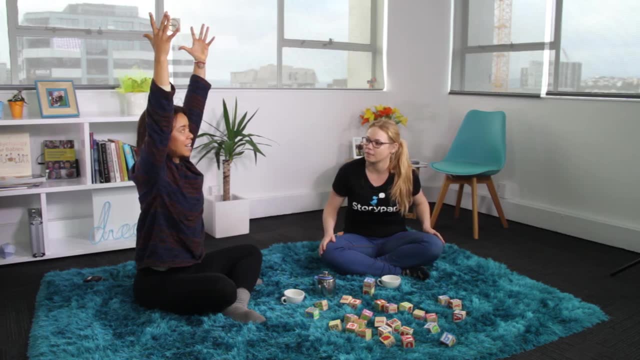 I think a really good one to start with is like always having your arms overhead and I'd say kind of growing like a tree right, and then having them look up at the hands and then exhaling. and why I do this posture is because it's simple, for 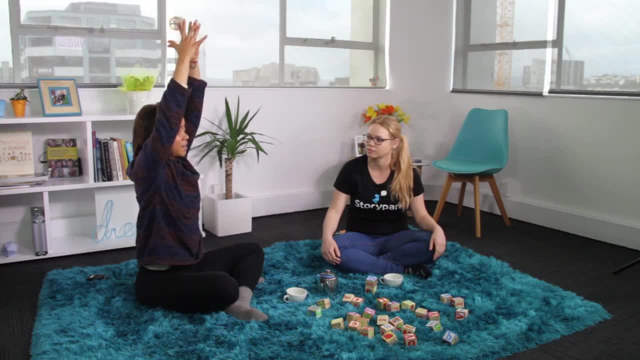 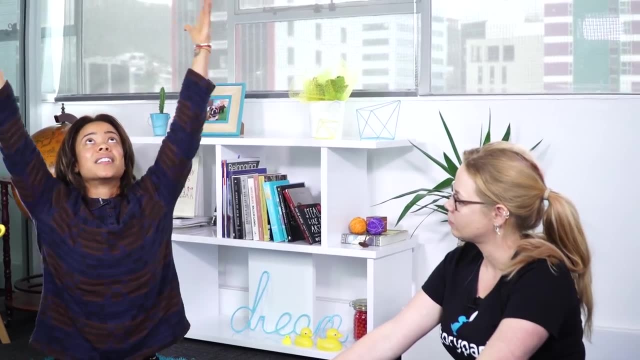 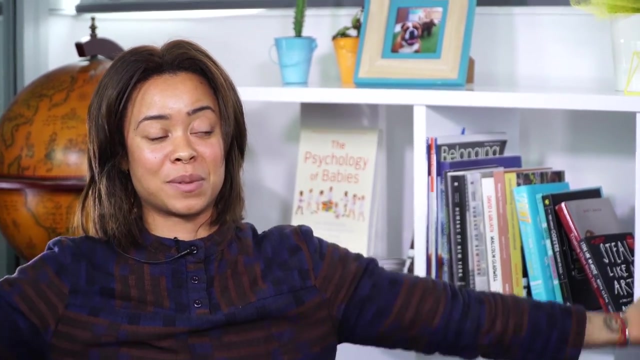 them to do and it's really important, right. so it kind of gets them: I, you inhale as the arms come up and then exhale as the arms come down. inhale and exhale, right, so they start to get into that idea of breath every time their arms move up and then from there having 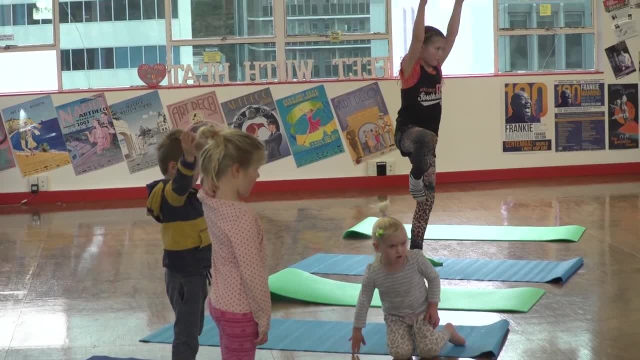 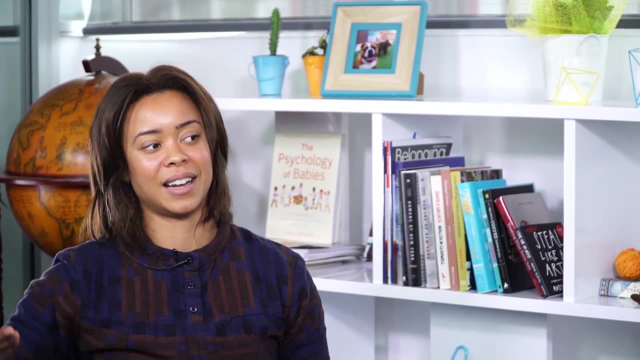 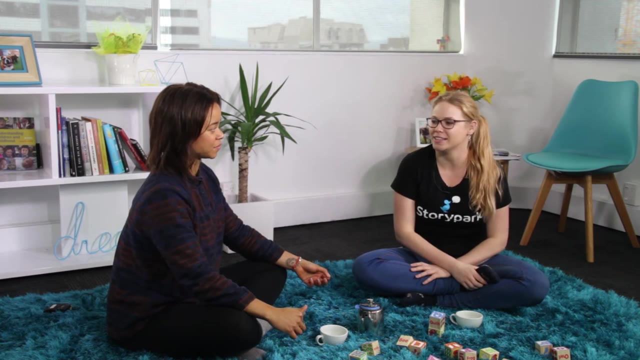 them hold that and like growing like a tree, and then we grow from there, like in terms of picking up the leg and and just like that, but having something moving with the breath, okay, and then building onto that. Kindergarten's are quite hectic, you know there's a lot going on. does that matter?